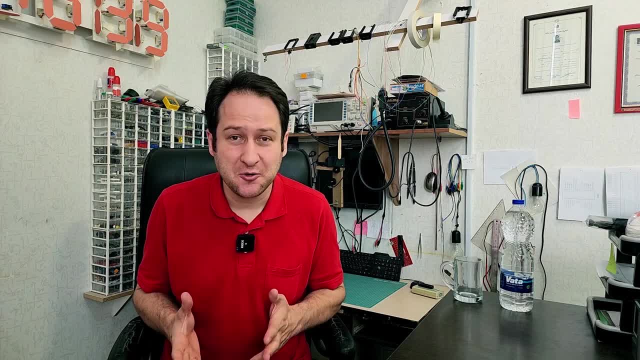 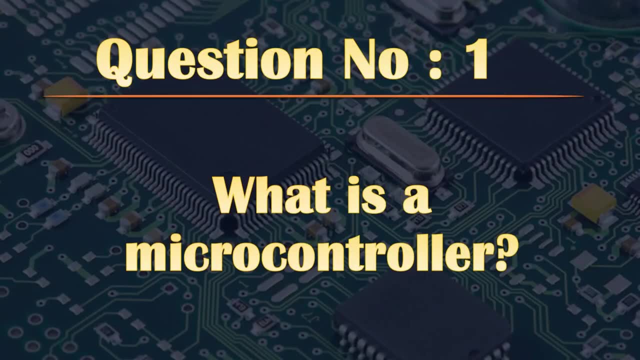 We are here to answer questions about microcontrollers, So the first question can be the Microc container itself, Question number 1.. What is a microcontroller? A microcontroller, also called an MCU or Microcontroller Unit, is an computer with multiple control system and 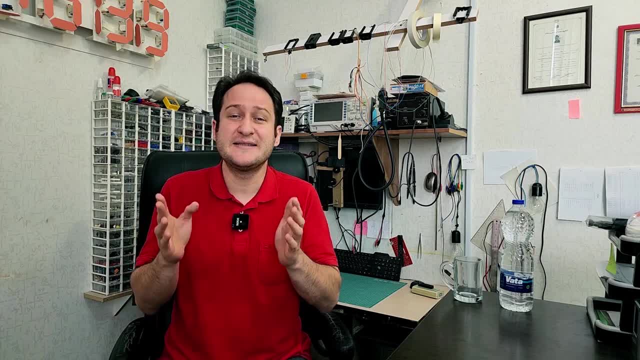 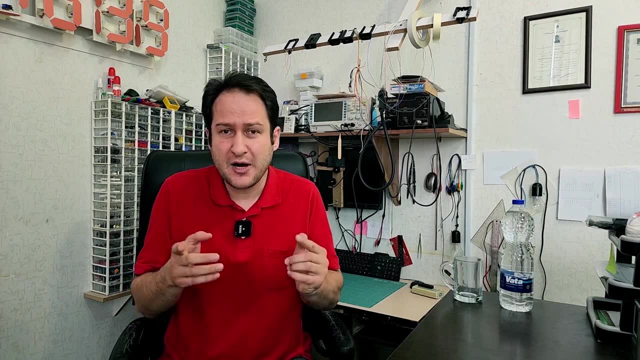 That's what they called a MC macros- hydraulics- and called MC macros an electronic chip. It's a small computer on a single VLSI integrated circuit that can execute codes and commands you write for it. A microcontroller contains components like CPUs. 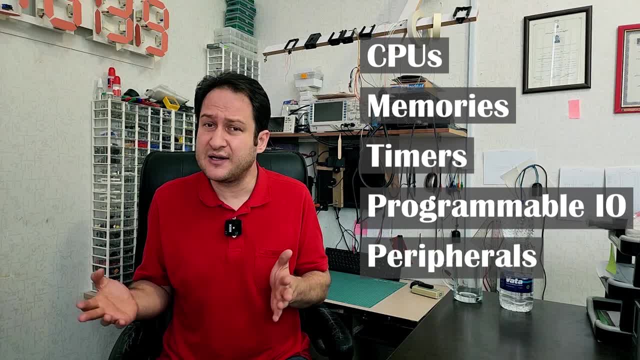 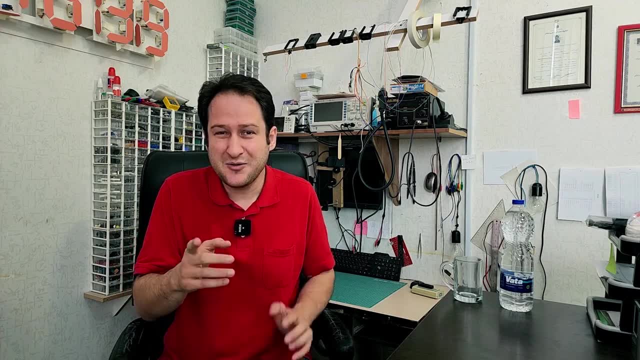 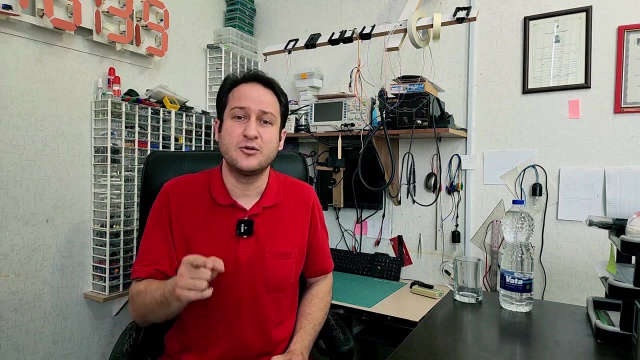 memories, timers, programmable IO peripherals, etc. In short, a microcontroller is a chip that can be programmed to do what you want. You can configure every single GPIO pin on a microcontroller to turn on or off in exact moment you define for it. Let's see some examples. These ICs are PIC MCUs. 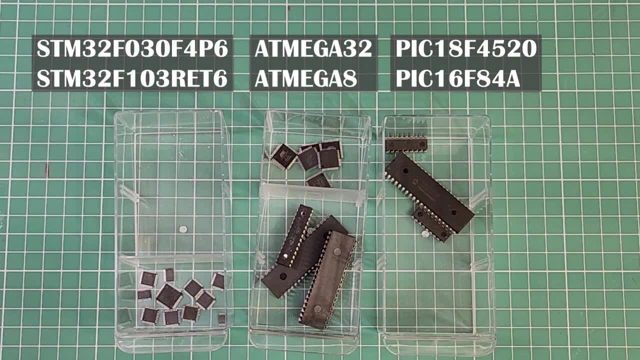 these are AVRs and these are STM32 microcontroller chips, each of which has its own characteristics, benefits and drawbacks, and, of course, each of them needs special tools and software. I will talk more about these differences later in this video. You may have heard of microprocessors, right? 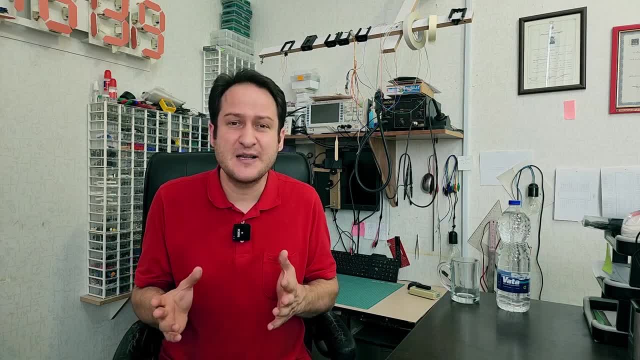 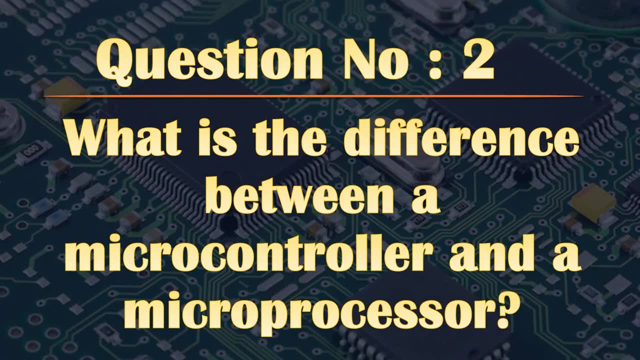 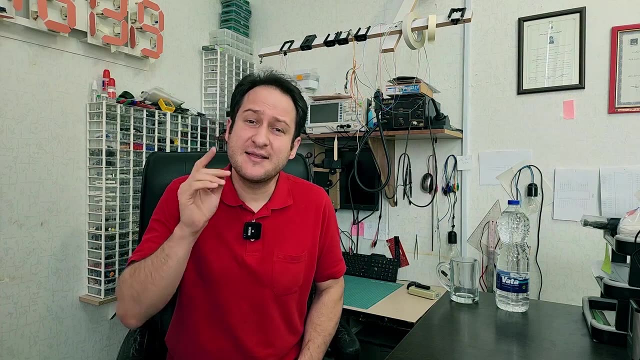 Sometimes my students ask me about the difference between a microprocessor and a microcontroller. This is a good question. Question number two: what is the difference between a microprocessor and a microprocessor? These two things are quite different. In short, there is at least one. 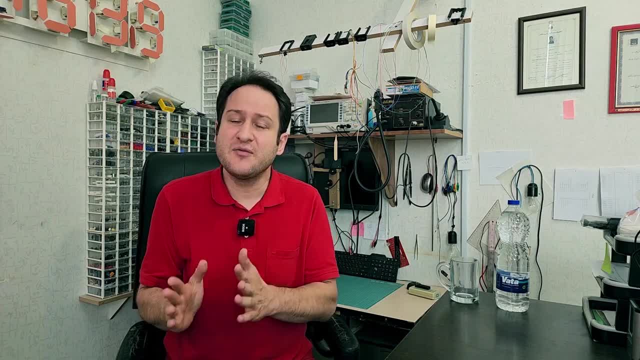 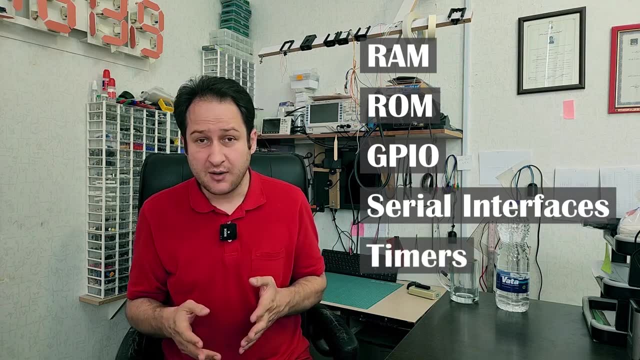 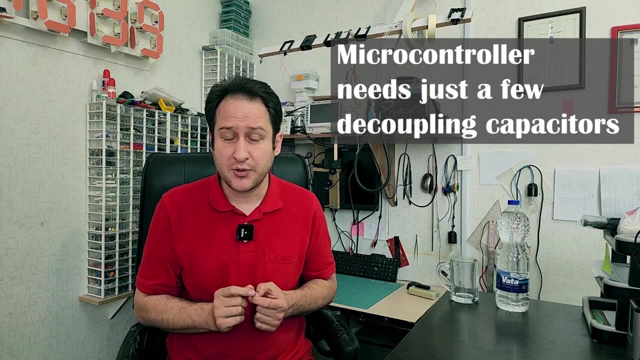 microprocessor inside a microprocessor, along with other stuff like RAM, RAM, GPIO, serial communication interfaces, timers, etc. In fact, a microprocessor is a chip that can be programmed to a chip that can operate alone with a few external components. but a microprocessor needs much more. 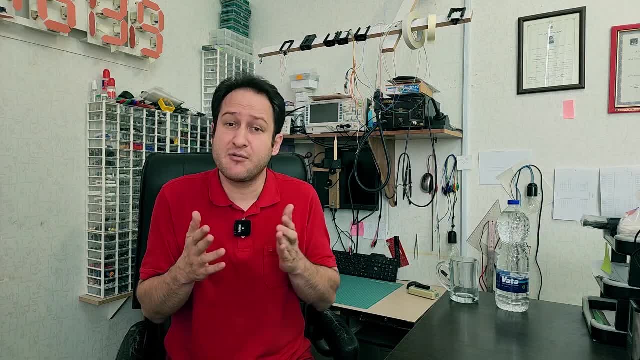 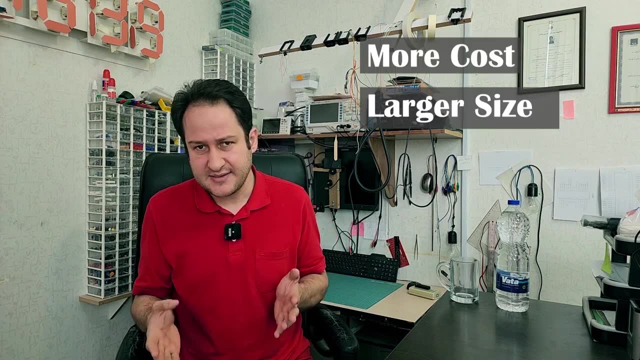 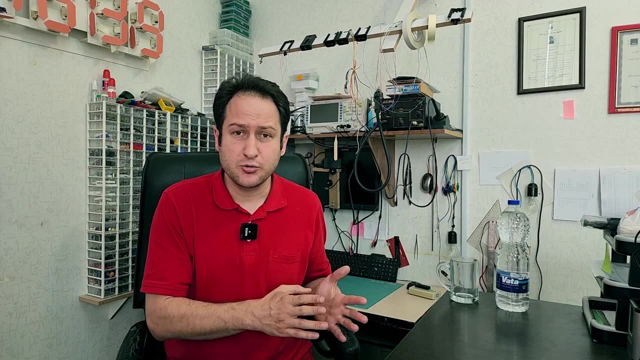 external components and ICs like RAM and ROM chips to become operational. More external components means more cost, a larger size, more power consumption and much more complexity. Now that the difference between a microcontroller and microprocessor become clear, you may ask me for. reasons to explain. I will explain in a little bit. First I will explain the difference between a microprocessor and a microprocessor. The difference between a microprocessor and a microprocessor is that the chip that operates alone, with a few external components, but a microprocessor needs. 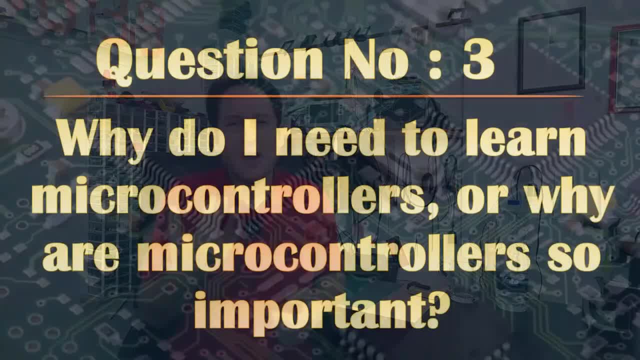 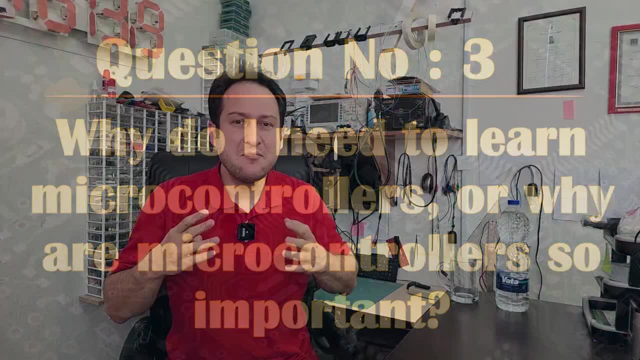 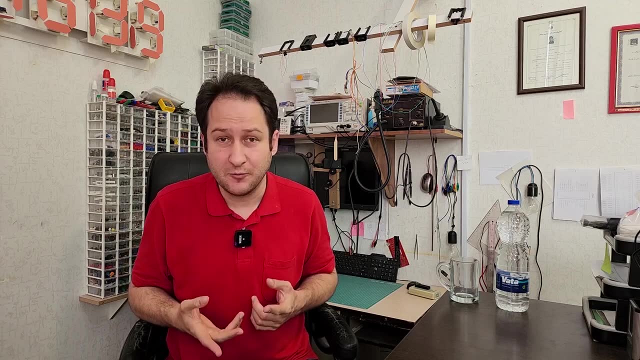 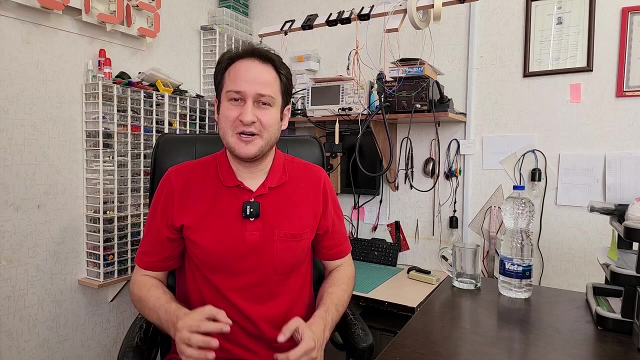 learn microcontrollers. question number three: why do i need to learn microcontrollers or why microcontrollers are so important? there are many reasons to learn microcontrollers. here i will mention four main reasons from my own point of view. reason number one: using microcontrollers makes things easier, even though learning a microcontroller or a programming language is 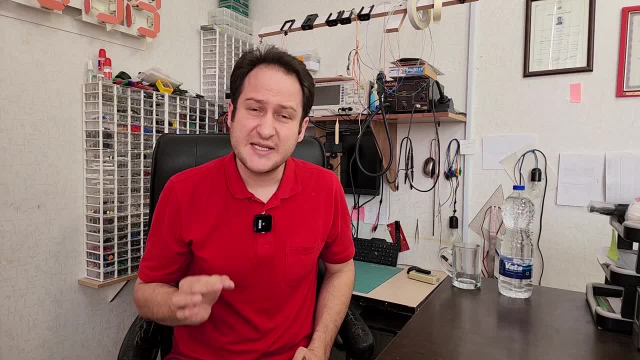 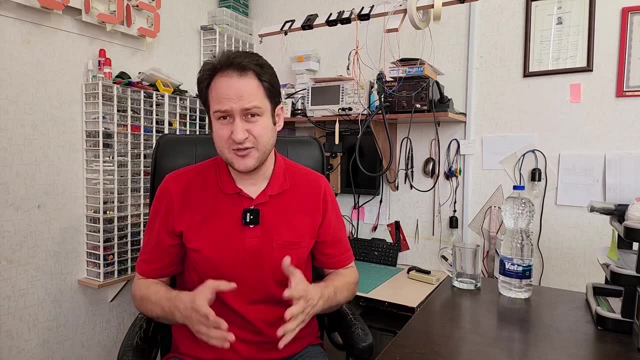 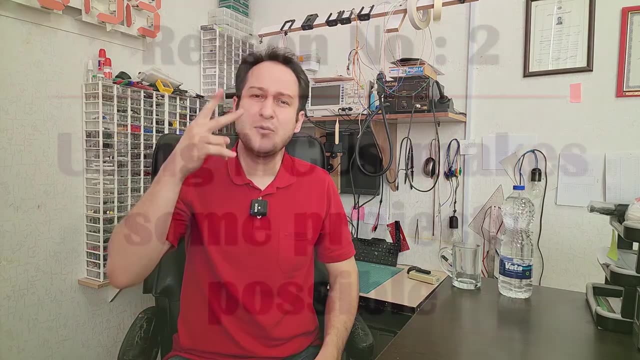 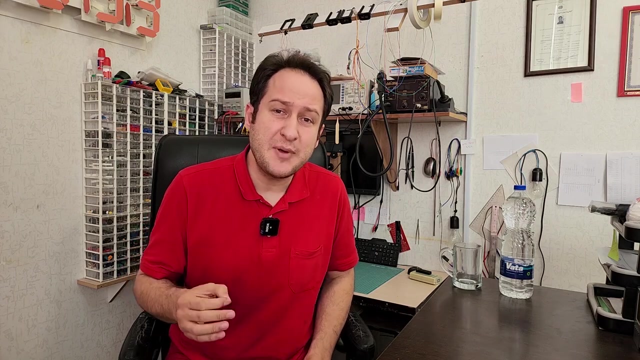 relatively difficult. it will make many problems easy to solve after learning them. after learning microcontrollers, you will prefer to make projects using microcontrollers instead of basic components, even a simple blinking led. reason number two: using mcus makes some projects possible. electronic projects these days are mostly based on modules like gsm module, bluetooth, lcd, glcd. 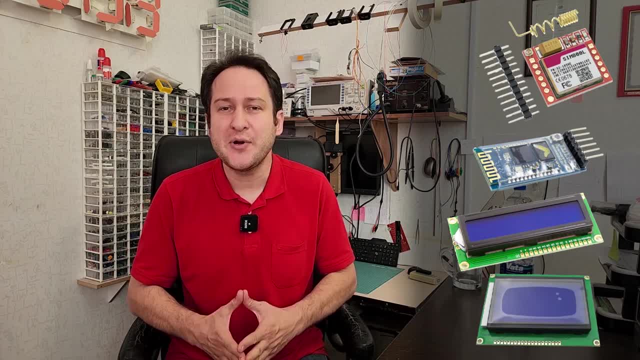 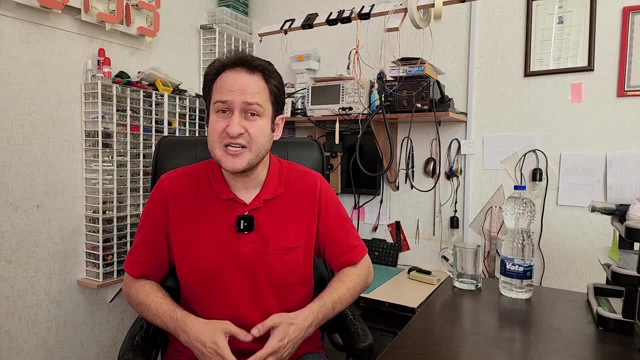 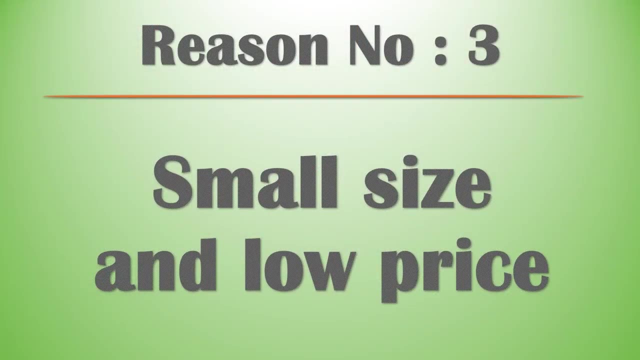 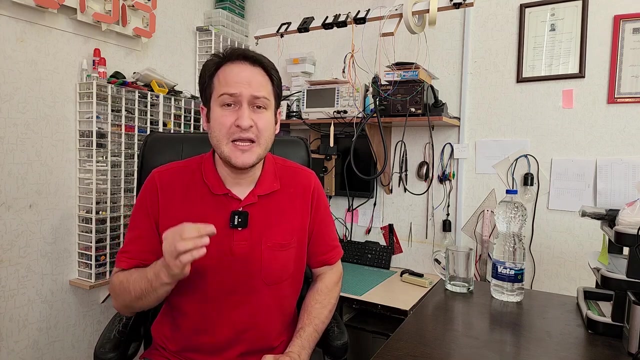 etc. most of these modules can't operate without commands from processors or microcontrollers, so using these modules in your projects without a microcontroller is almost impossible. reason number three: small size and low price. microcontrollers are much smaller and cheaper compared to any other computer system. if you intend to use a computer system in your project. 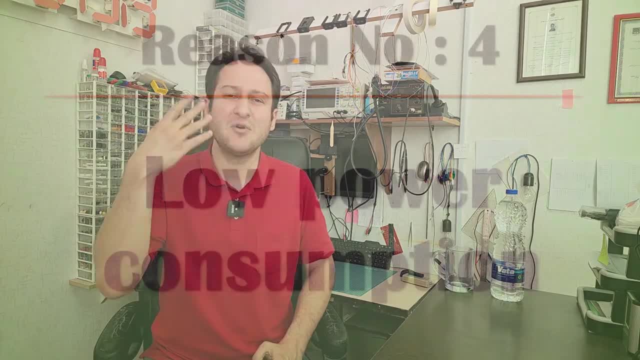 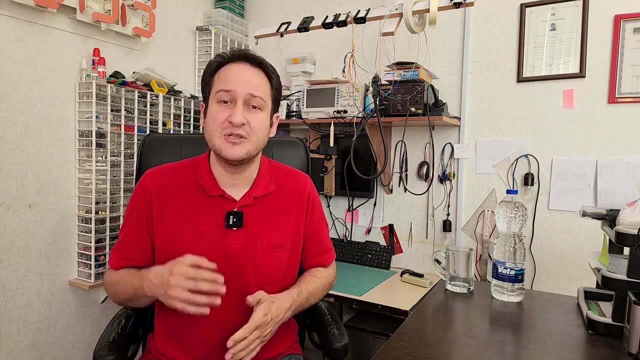 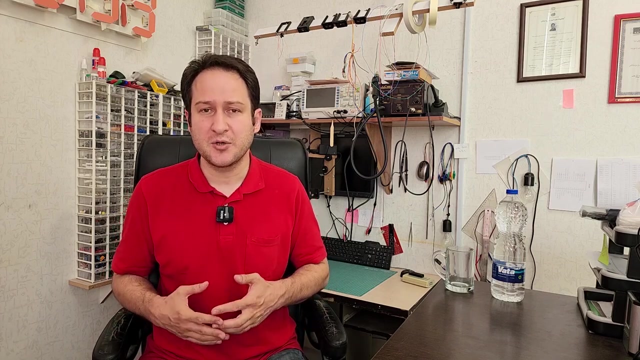 using a microcontroller will be a good choice. reason number four: low power consumption. it is very important, especially in a battery-powered device that needs to last for a long period of time. microcontrollers consume much less power compared to any other computer system. these are main reasons for learning micro. 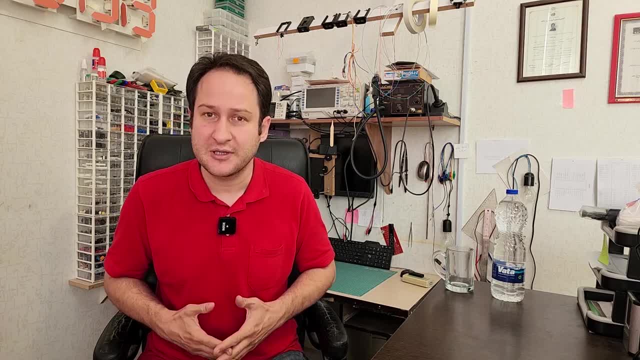 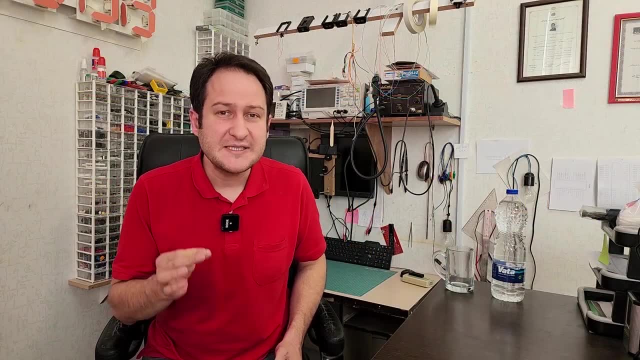 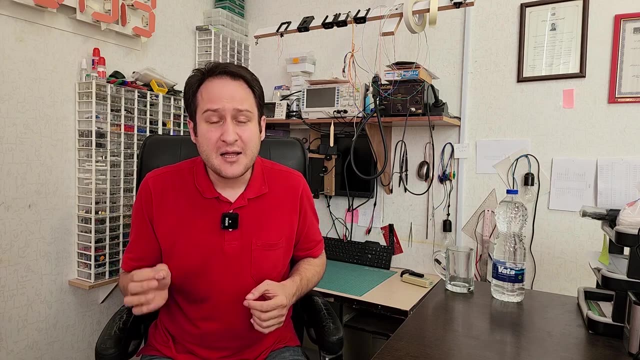 controllers. now that we are combined to learn microcontrollers, the next question is question number four. where should i start from? in my opinion, the very first step in learning my microcontrollers is to select the mcu family. you are going to learn there are a lot of mcu families. 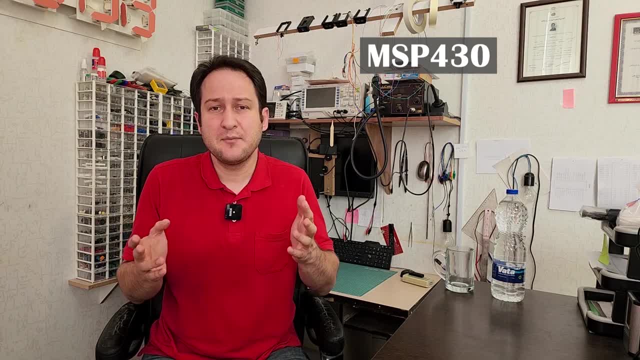 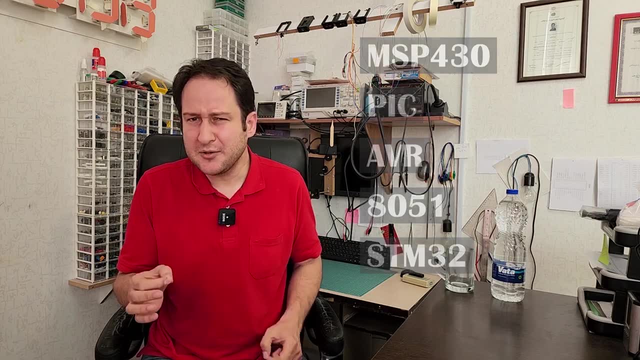 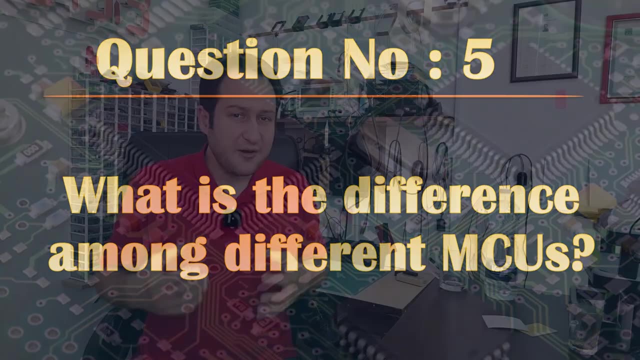 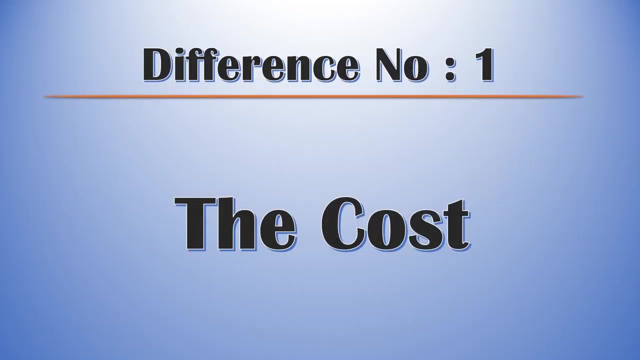 on the market, like msp413, pic, avr 1851, stm32 arm series, etc. here you may ask question number five: what is the difference among different mcu chips and mcu families? there are a lot of differences among different mcus. here i'm going to mention nine of them. difference number one: the cost. some 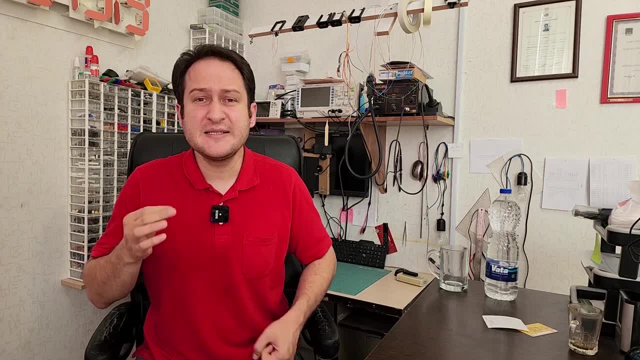 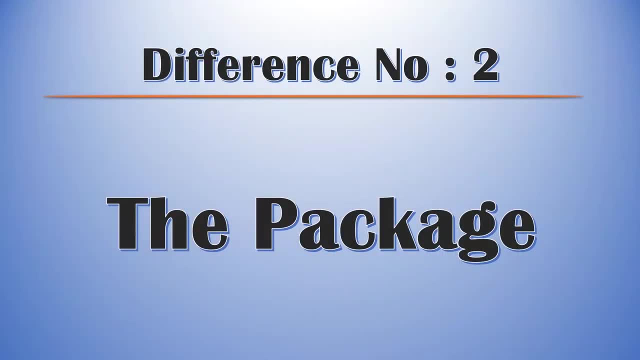 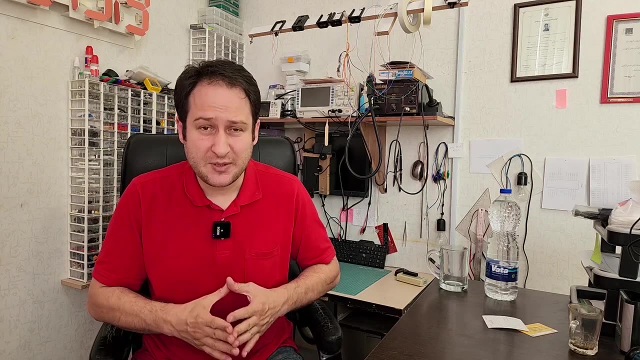 microcontrollers are expensive and some are cheap. this is one of most important factors in selecting right microcontroller for a project. difference number two: the package. most of microcontrollers are available only in deep packages or only in smd packages, but you can find some microcontrollers. which are available in both smd and mcu families so you can find some microcontrollers which are different in smd and deep packages. difference number three: memory size and type. usually mcus have several memory types, for example ram, flash and e2p ram are the most common memory types in mcus. 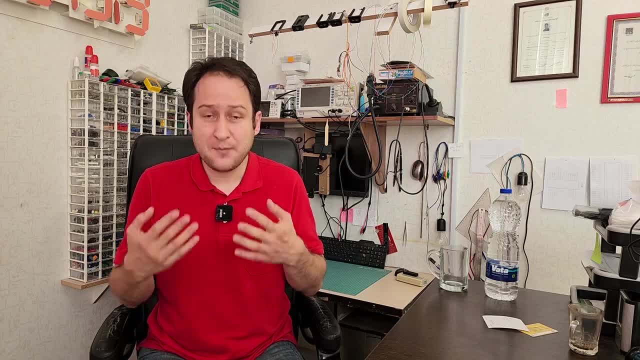 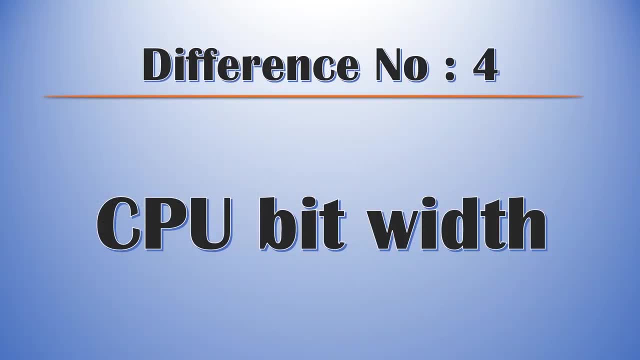 it is obvious: the more memory a microcontroller has, the better. microcontrollers with large memory size are expensive, though. difference number four: cpu bit width. another difference is in their cpu bit width. you can find 8 bit, 16 bit and 11 bit. you can find 8 bit, 16 bit and 11 bit. 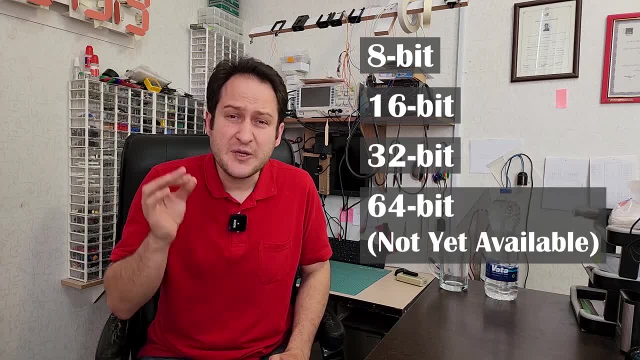 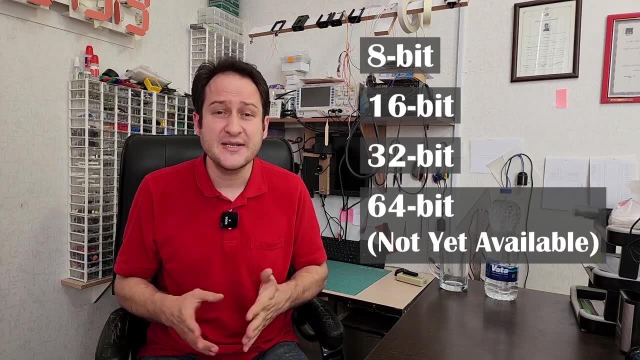 you can find 8 bit, 16 bit and 11 bit, 32-bit and even 64-bit-wide microcontrollers on the market. These numbers show the quantity of bits a CPU can process at a time or in a single clock pulse. 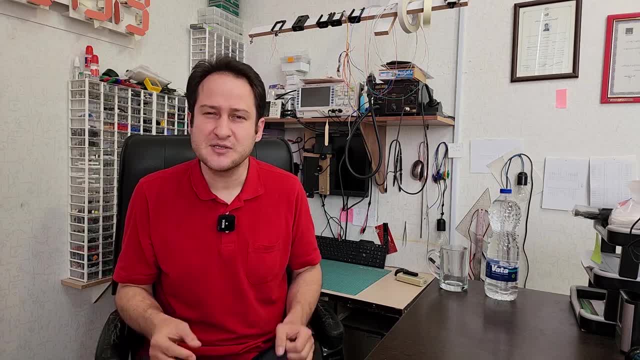 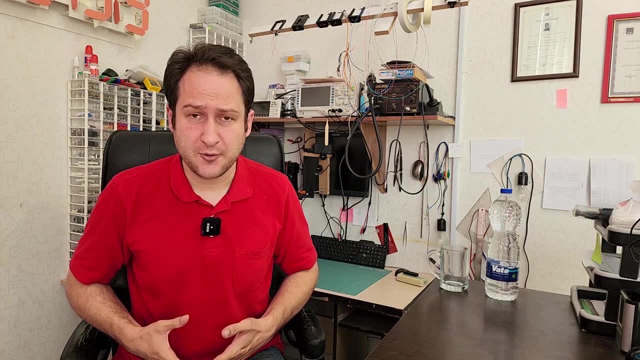 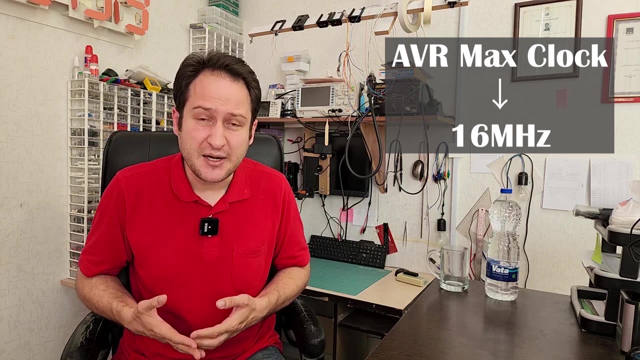 The wider the CPU bit, the better and, of course, the more expensive. Difference number five: max clock speed. Max clock speed differs in different microcontrollers. For example, AVR microcontrollers can operate at a maximum frequency of 60 megahertz, while 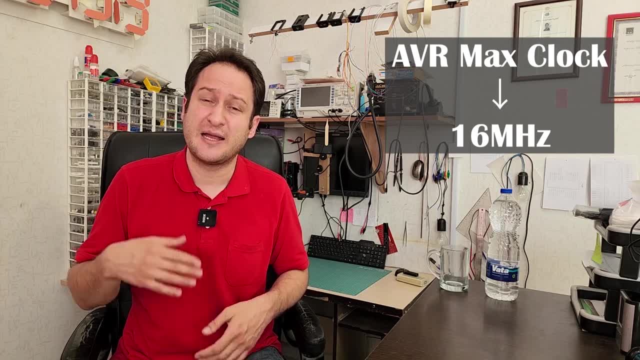 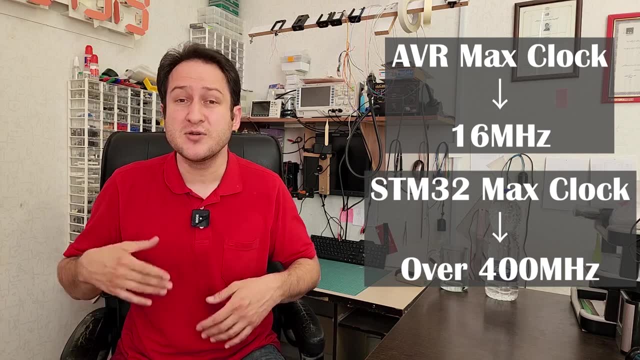 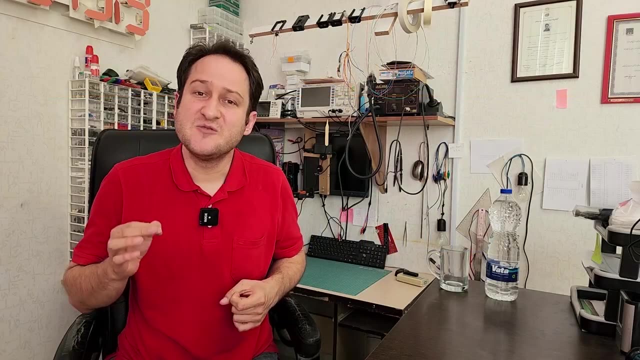 some STM32 microcontrollers can operate at more than 400 megahertz. It goes without saying that more frequency means more CPU power and, of course, more price Difference. number six: GPIO pins. GPIO pin count is one of the most important factors in selecting the right MCU for a microcontroller. 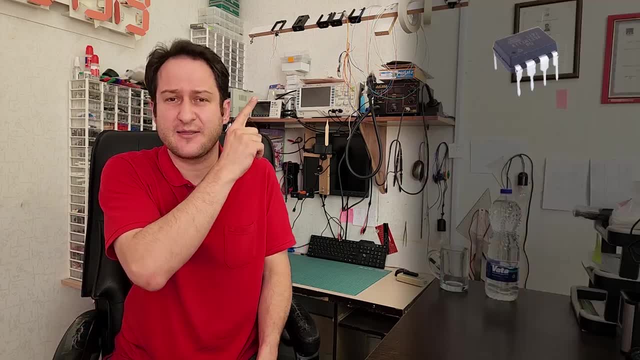 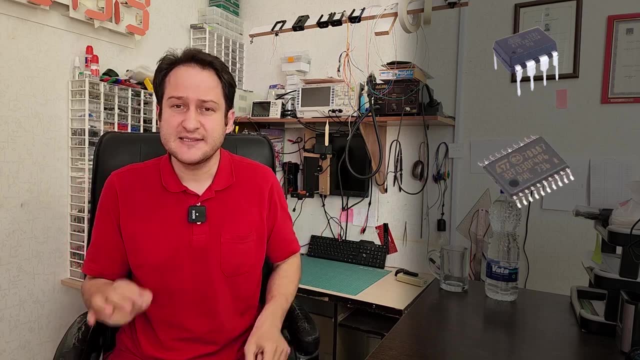 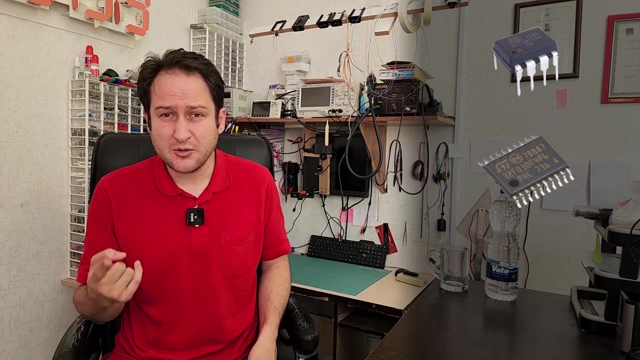 For example, this Atiny13 AVR microcontroller has 6 GPIO pins, while this STM32F030F4P6 microcontroller has 13 GPIO pins. I mean you can connect more external devices to this STM32 compared to this AVR. 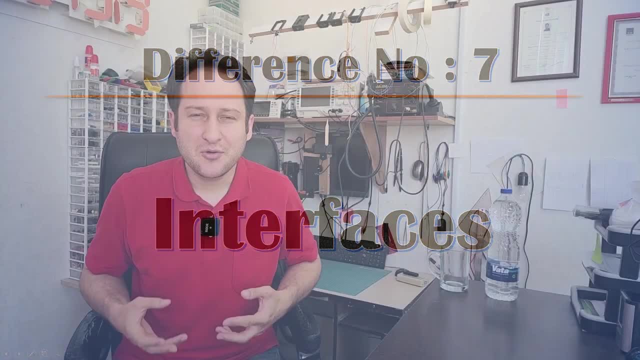 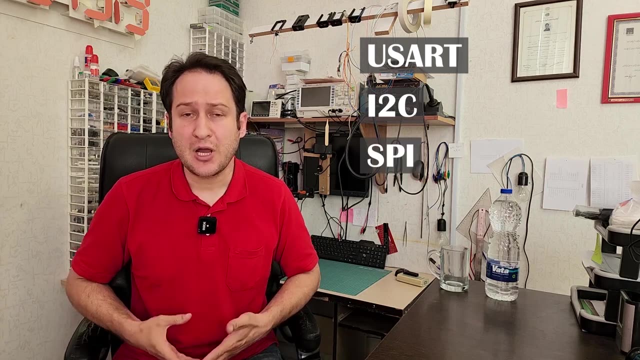 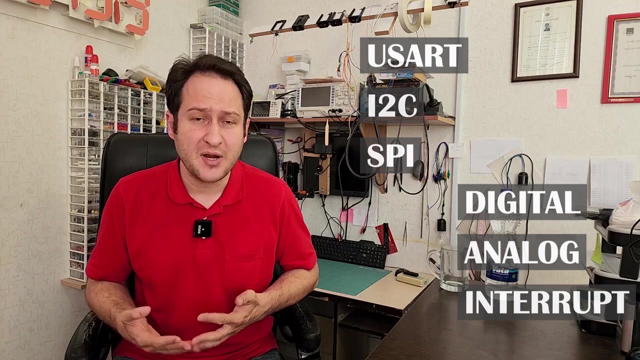 Difference number seven interfaces it supports. Each microcontroller supports a few protocols, Like USART, I2C, SPI, etc. and a few input type like digital input, analog input, external interrupts, you name it. It is different on different microcontrollers. 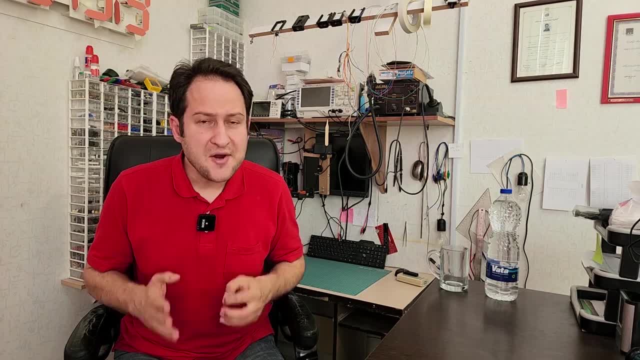 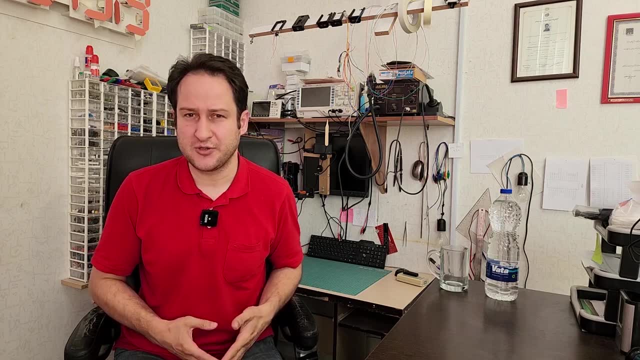 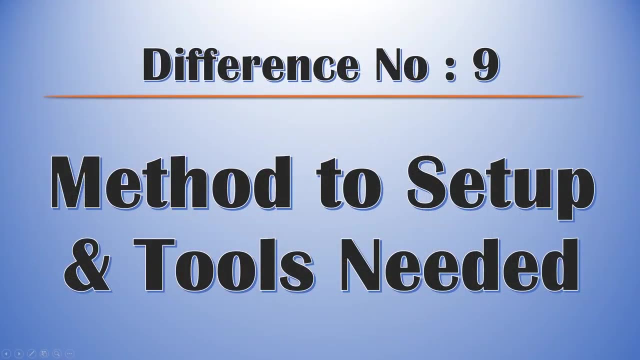 Difference number eight: sensitivity to noise. Almost all microcontrollers are sensitive to noise, but the amount of this sensitivity is different for different microcontrollers. Usually, deep packaged microcontrollers are less sensitive to noise. Difference number nine: method to set up and tools needed to configure. 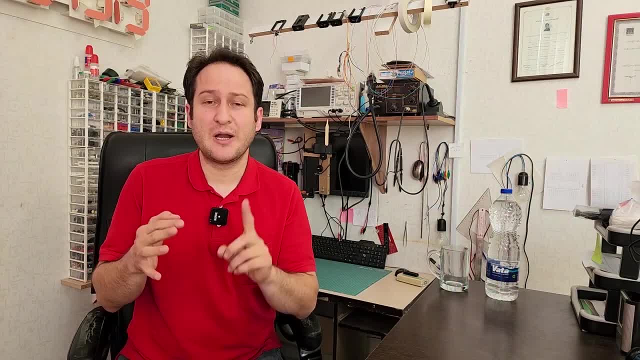 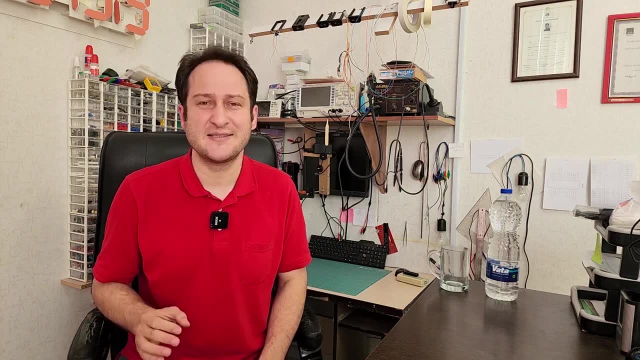 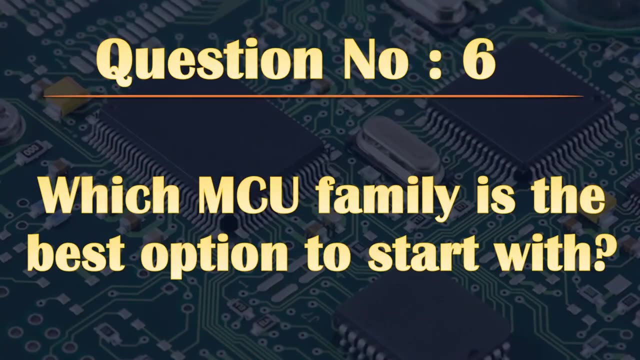 Each MCU family has its own programmer software, programmer device and compiler software. To work with a particular MCU family you have to learn specialized software. So at this stage we are facing next question, Question number six: which MCU family is the best option to start with? 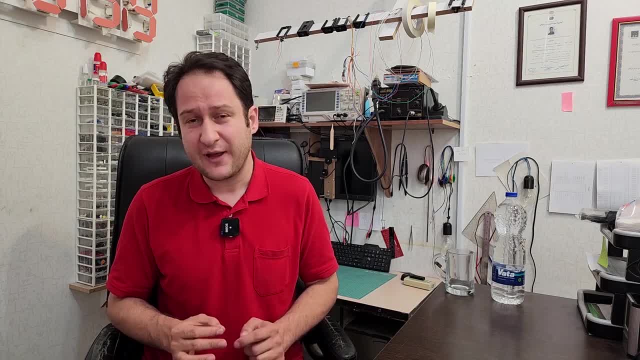 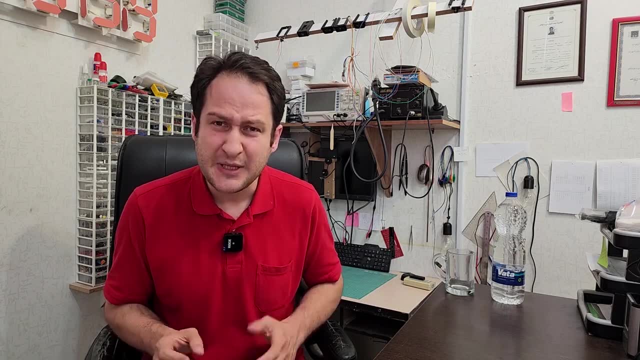 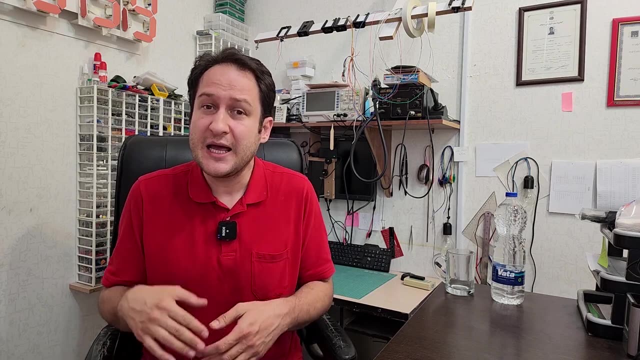 There is no special rule for selecting your very first MCU family, But I recommend this one, Starting with a deep packaged MCU. Deep packaged MCUs don't need PCB and you can run your first projects on a breadboard. This will help you improve your microcontroller and programming skills very quickly. 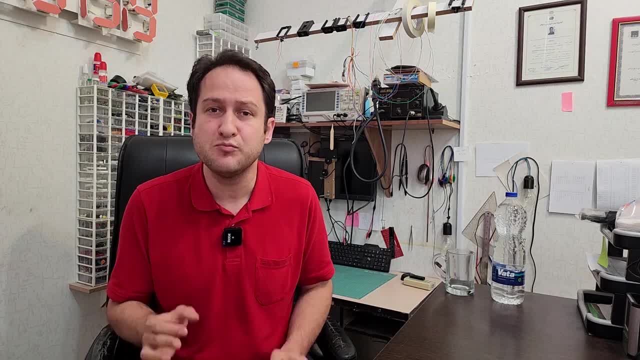 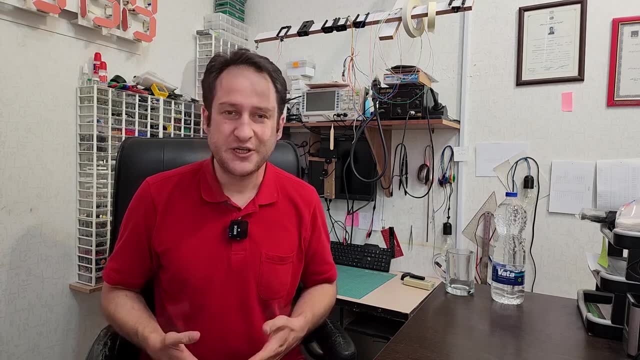 In addition, a deep packaged MCU resists noise much better compared to SMD packaged MCUs. This will guide you through your first steps on your journey. On the other hand, I recommend starting with an easy microcontroller. I recommend starting with an easy microcontroller. 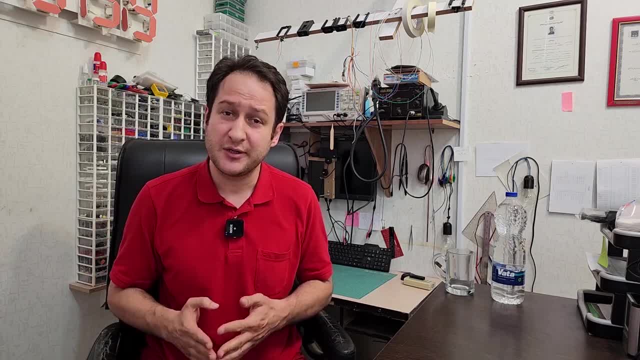 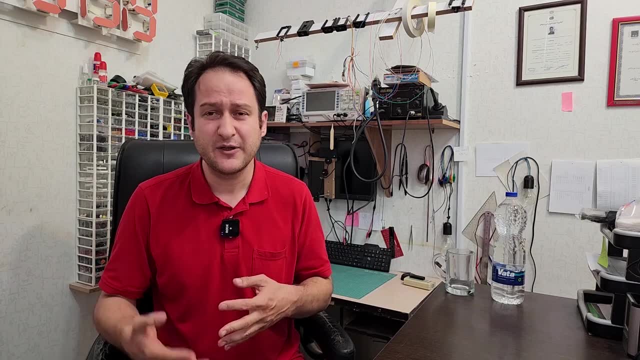 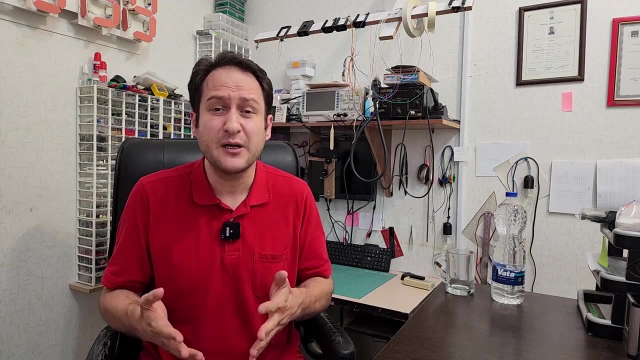 I recommend starting with an easy microcontroller. An easy to learn microcontroller will motivate you to continue learning microcontrollers, Since process of setting up and configuring microcontrollers is very similar. learning an easy microcontroller will help you to learn difficult microcontrollers easily. 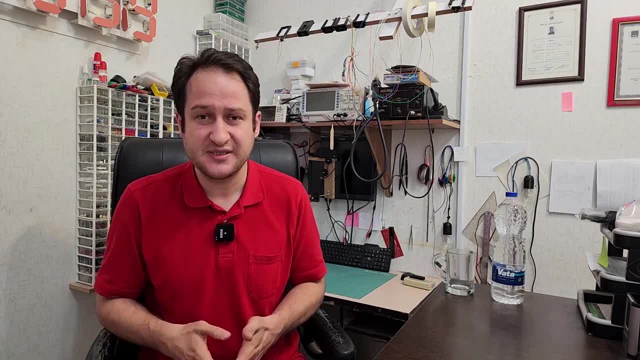 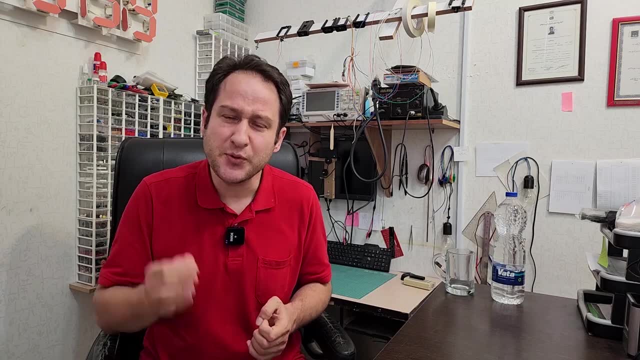 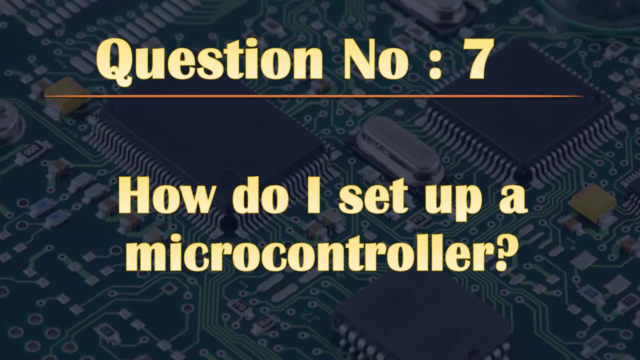 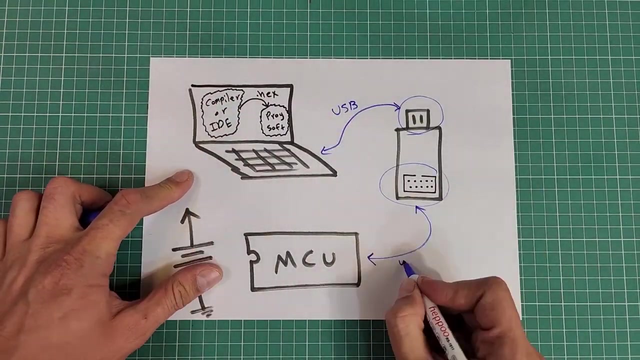 I think PIC or AVR are good options. I started with AVR and I think it was a good choice. It has deep packages. It is super easy to learn. Now is the time to answer next question, Question number 7.. How do I set up a microcontroller? 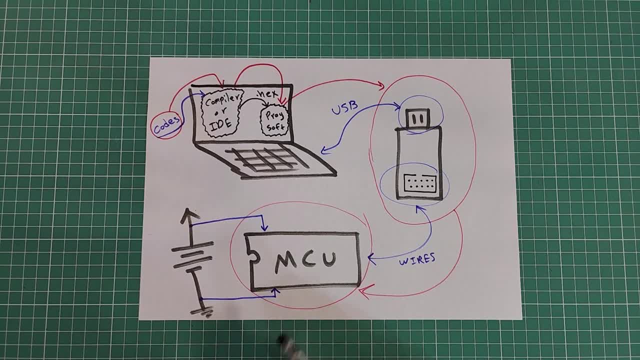 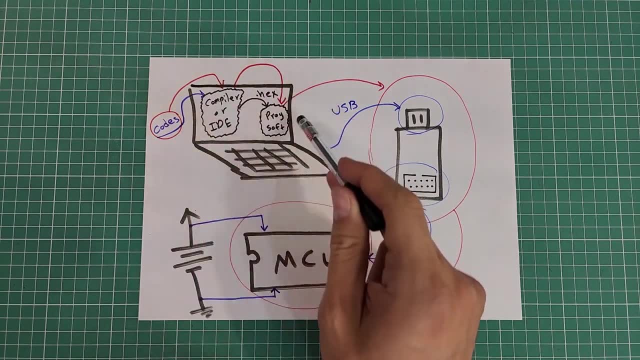 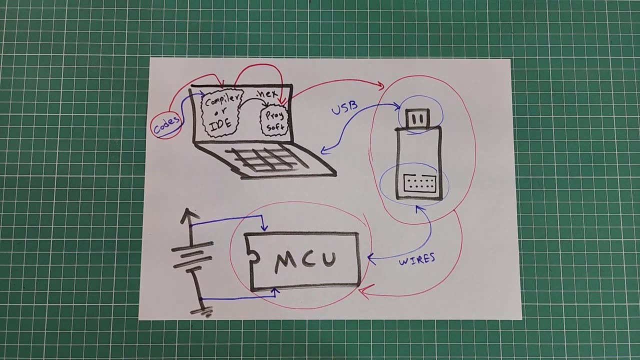 In order for a microcontroller to work, we need to set it up and program it. This process is common among all microcontroller families. You need a computer and a computer, The compiler software installed on it, to write codes into it and make an executable file. 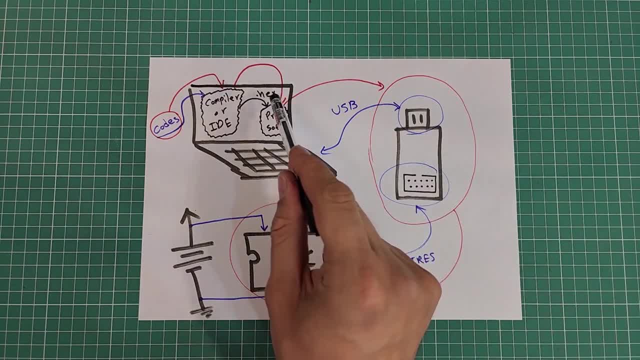 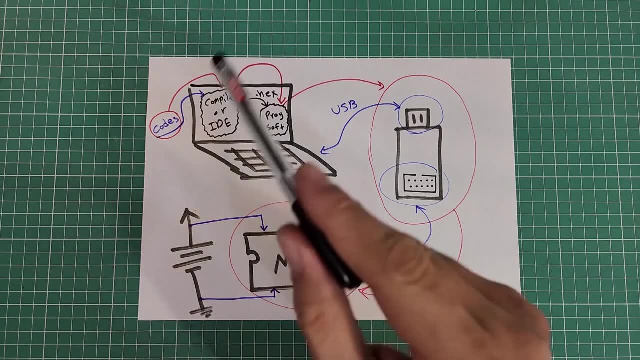 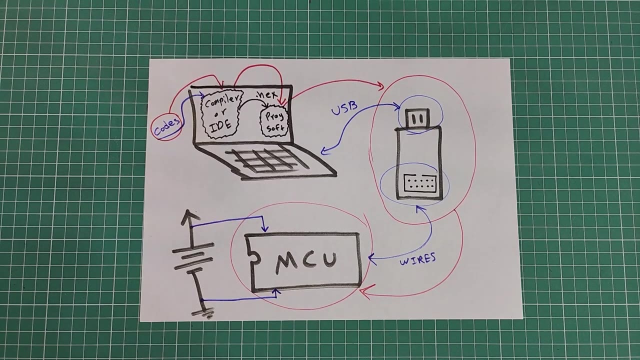 You also need a programmer device and software on this computer to operate this programmer device, which I call it a programmer software. Sometimes the executable file is called hex file or hex file. This software is usually called an IDE or integrated development environment. 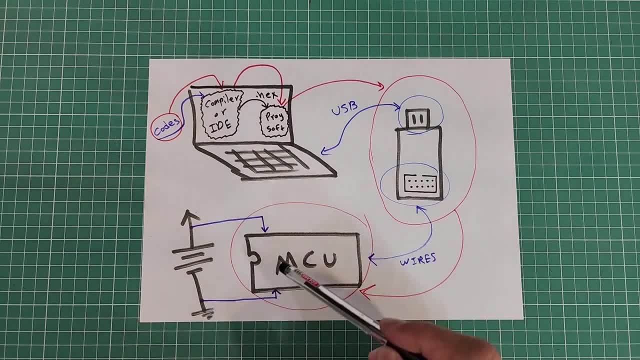 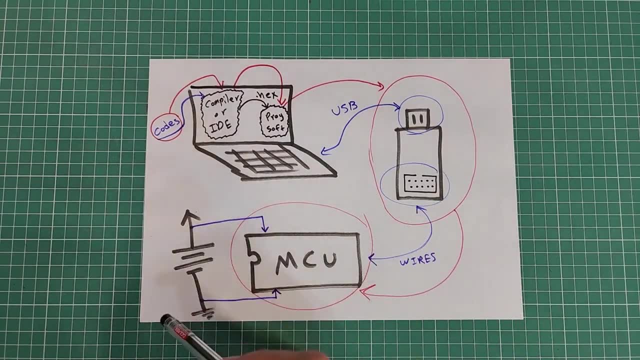 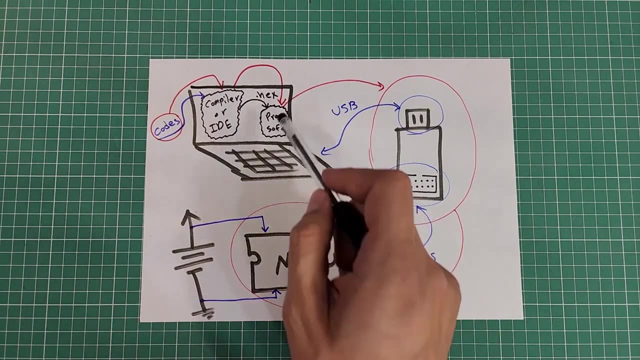 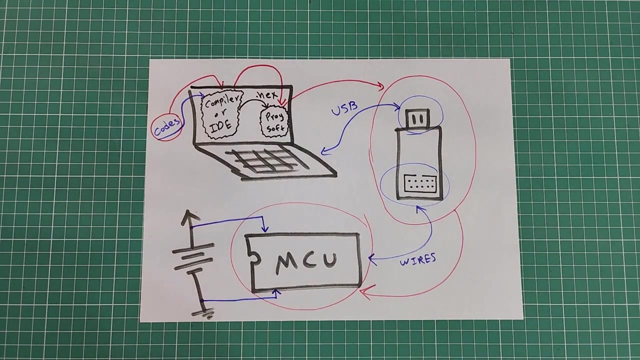 The process starts with this: In first step we have to write some codes here on this compiler software and then make an executable file from codes using this compiler software. Then we have to load hex file or executable file on the programmer software. The main job of programmer software and programmer device is to transfer executable file from. 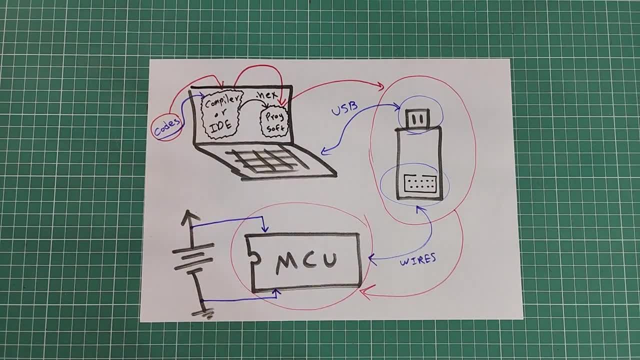 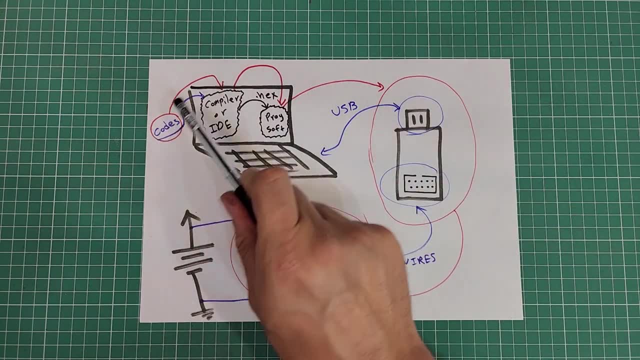 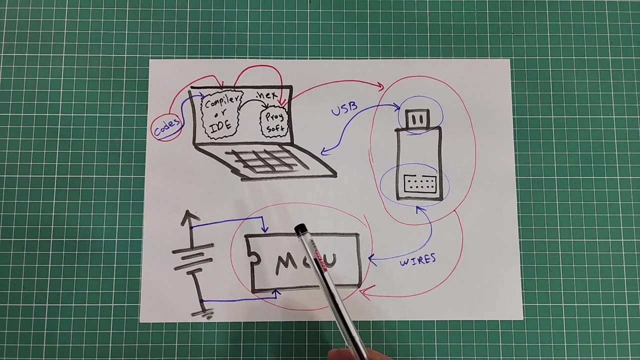 this computer into this chip. This process is called hex file, Sometimes it is called flashing or sometimes it is called programming. Sometimes this whole process from coding to flashing the microcontroller is called programming. And finally you need a power supply to power the chip up. 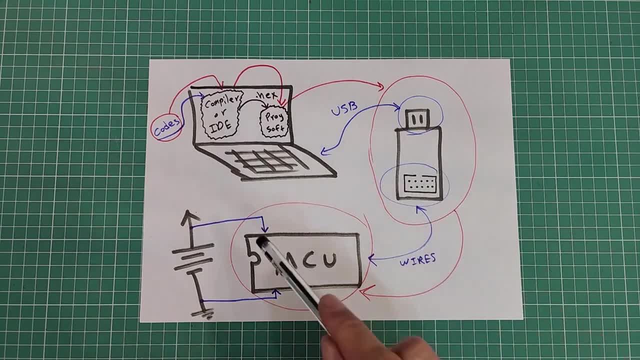 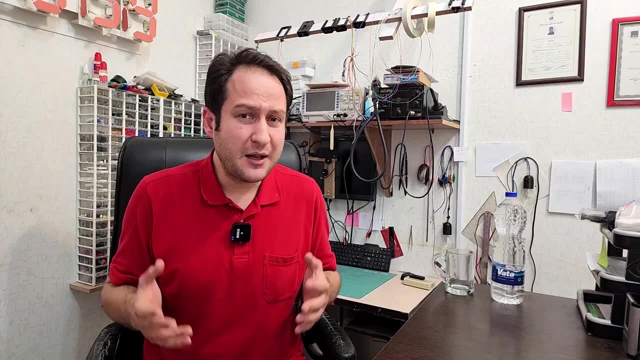 Otherwise the programmer device will fail to flash the microcontroller. Although some programmers don't need a power supply to flash a microcontroller, There are a lot of MCU families on the market. It is obvious All of those have their own microcontrollers. 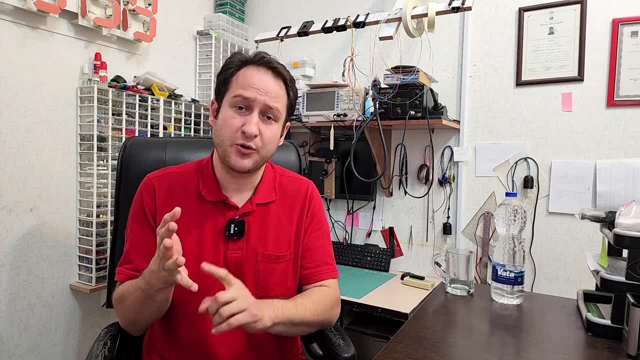 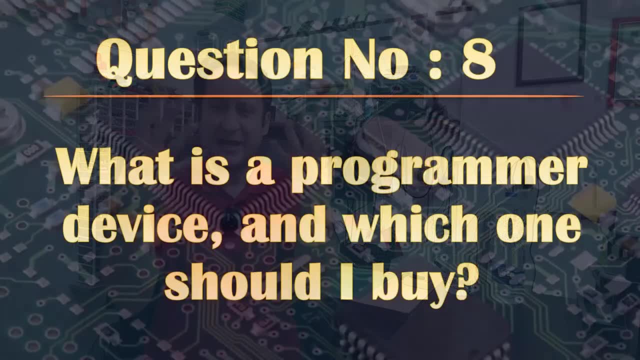 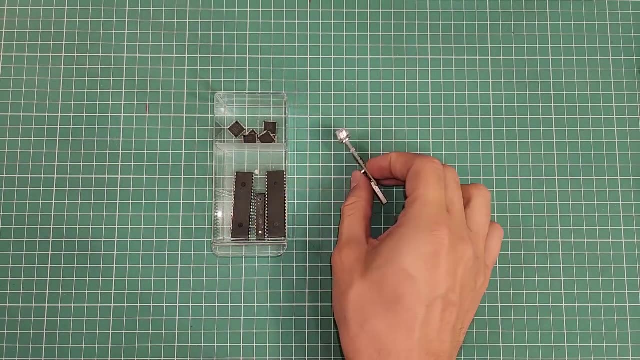 They have their own compiler software, programmer device, programmer software setup and configuration. So you may ask your last question, Question number 8.. What is a programmer device, and which one should I buy? These are AVR microcontrollers. This is one of programmers that can flash these MCUs. 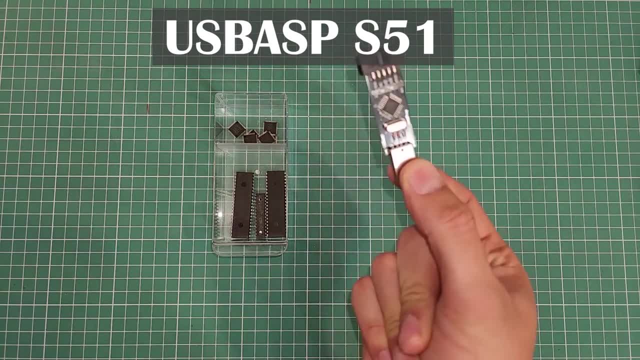 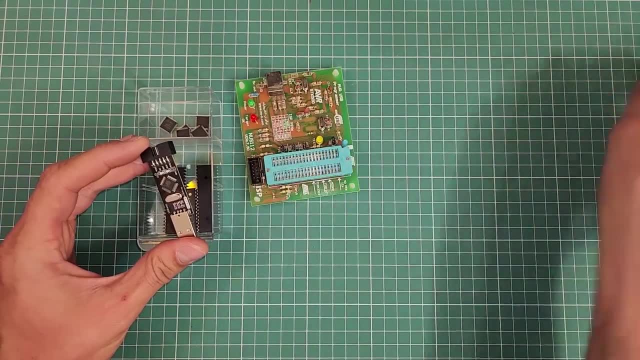 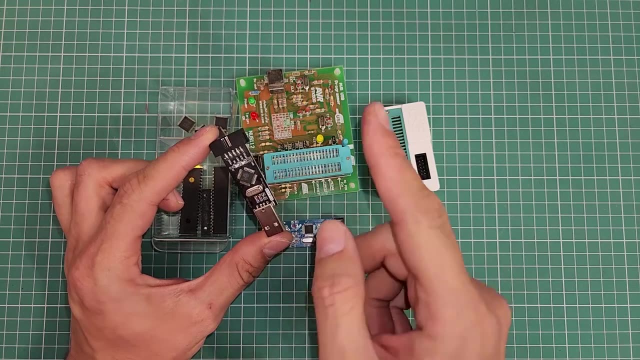 Its name is USB-ASB-S51 and it is available in online shops. There are other similar programmers out there Like this one, this one or this one. If you intend to work with AVR microcontrollers, I recommend buying a programmer like this. 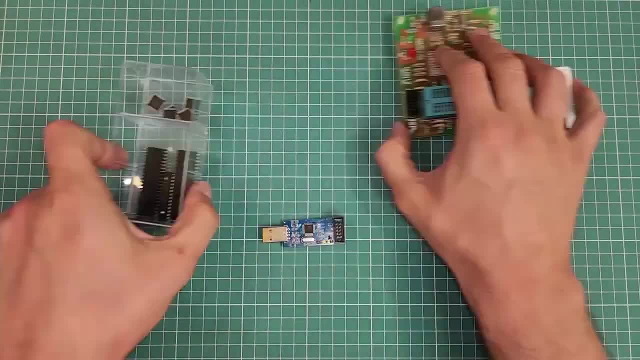 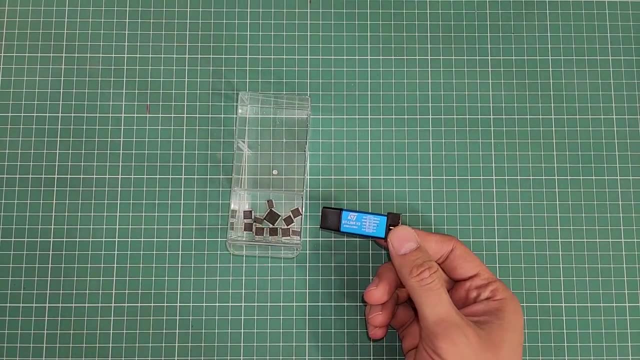 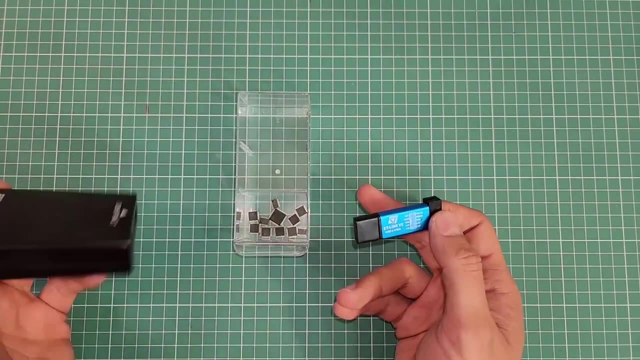 one. These are cheap and handy. This is an ST-Link programmer which can flash STM32 microcontrollers Also. I got this one which supports STM32 microcontrollers and some other MCUs. If you intend to use STM32 microcontrollers, I recommend buying this one. Also, I got this one which supports STM32 microcontrollers and some other MCUs. Again, if you intend to use STM32 microcontrollers, I recommend buying this one. Again, if you intend to use STM32 microcontrollers, I recommend buying this one. 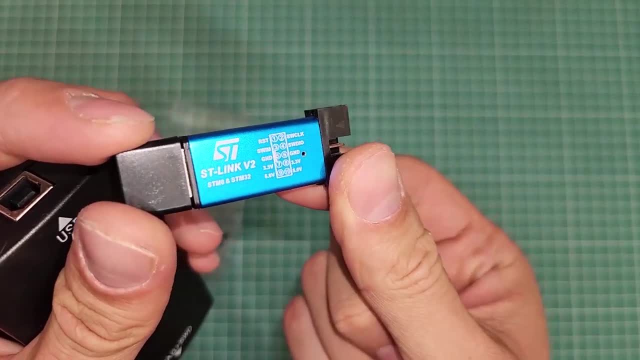 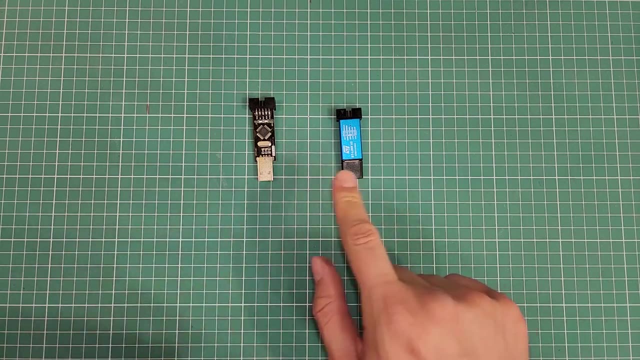 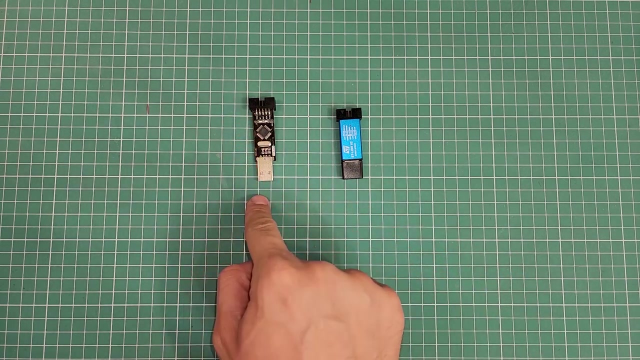 Again, if you intend to use STM32 microcontrollers, I recommend buying this one. This is a good choice. These two programmers are specialized for a certain MCU family. This one is for AVR flashing and this one is for STM32.. I mean, you can't use this one to flash an STM32 MCU or this one to flash an AVR. 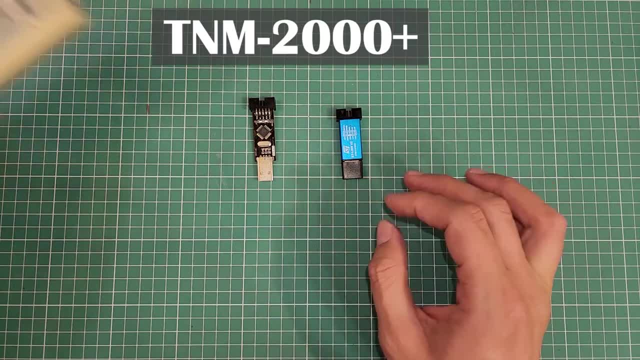 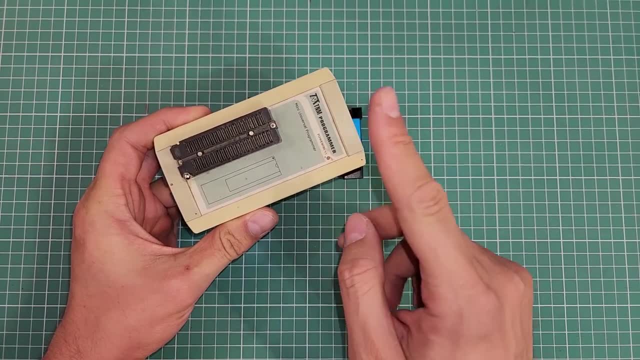 But if you buy a universal programmer like this TNN programmer, you can program it at any time as long as you want. However, it depends on the type and size of yourther program. many ICs using one programmer. For example, I am using this lovely TNM Universal. 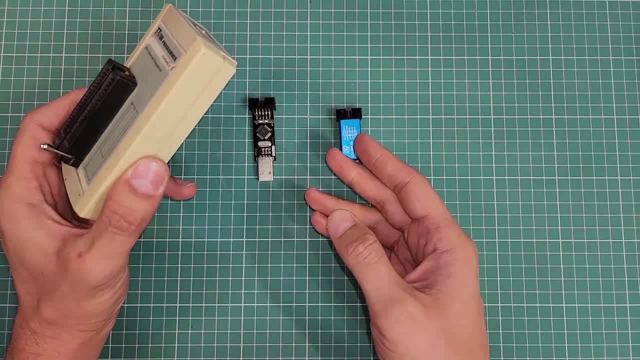 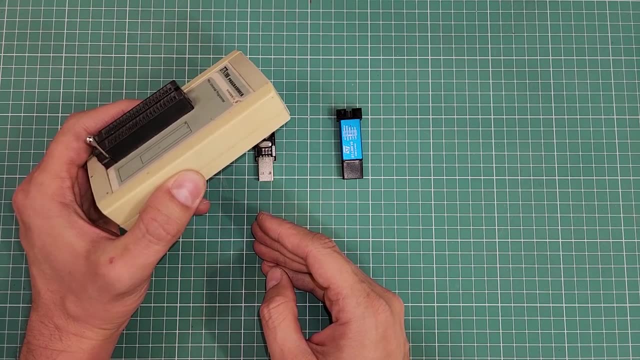 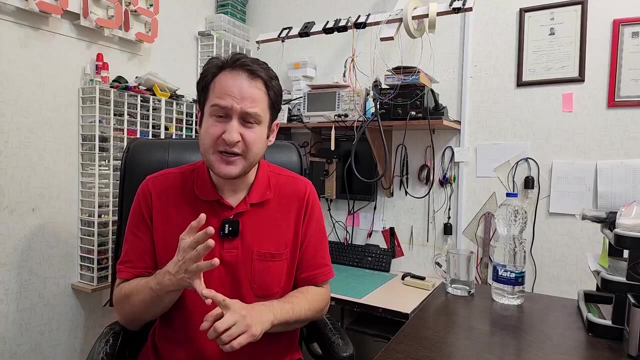 programmer to flash PIC, AVR and Atmel ARM microcontrollers, while there are special programmers for each of them. The last point here is to learn how to connect an MCU to a programmer. Every MCU family has its own programmer, software connection, setup and configuration. I can't. 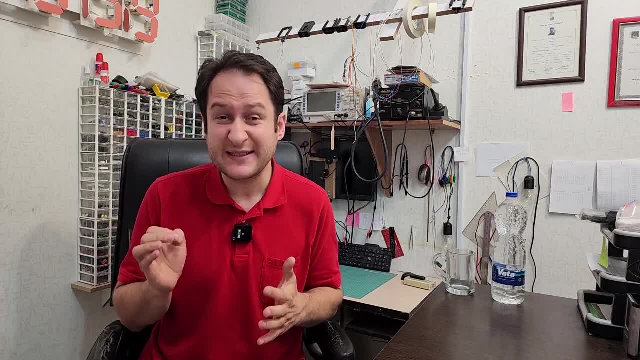 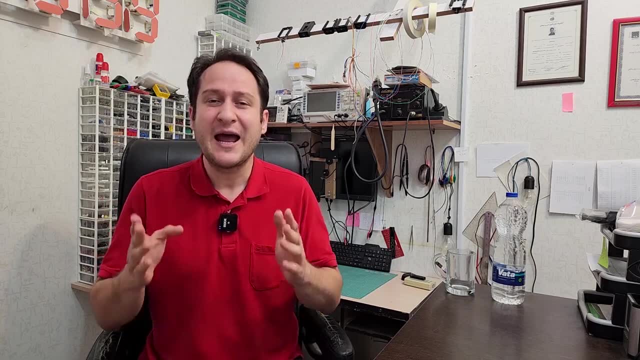 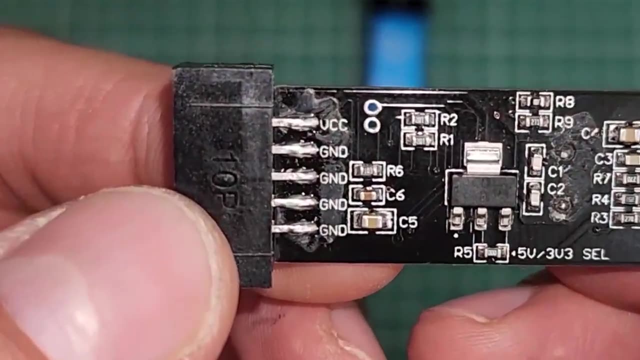 explain all of them here in this video. So I will explain them in exclusive videos for each microcontroller. For now it is enough to take a brief look at AVR and STM32 programmers. Let's look at these pins here: VCC, GND, GND, GND, GND. These are for power rails and 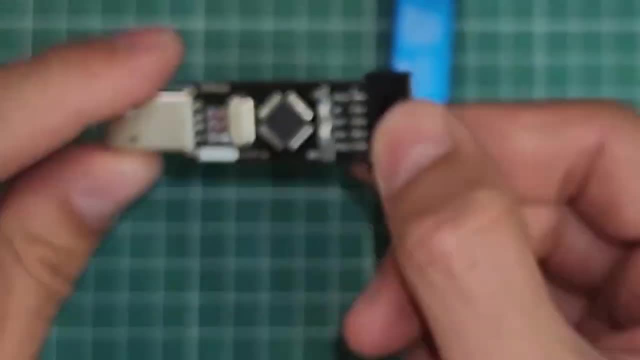 here: MOSI, RST, STK and MISO. These pins form the ISP port and almost every other ISP is connected to the power cable. This is the power cable of the PC. This is the power cable of the PC. This is the power cable of the PC. This is the power. 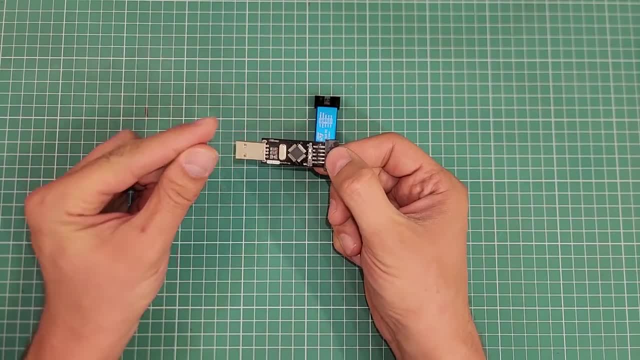 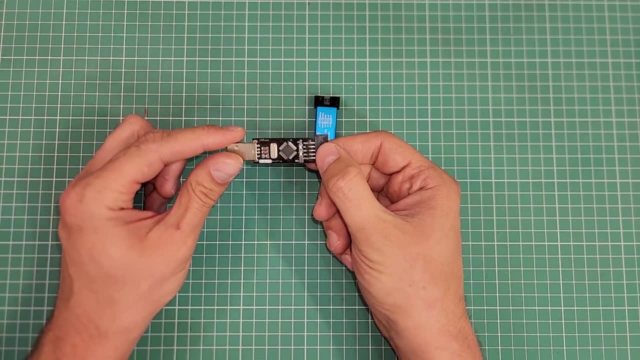 of the PC. This is the power cable of the PC. This is the power cable of the PC. This is AVR chip supported. If you look at any AVR MCU pinout, you can find similar pins on the chip. I will explain AVR microcontrollers in the next video. Let's look at this one. These are RST. 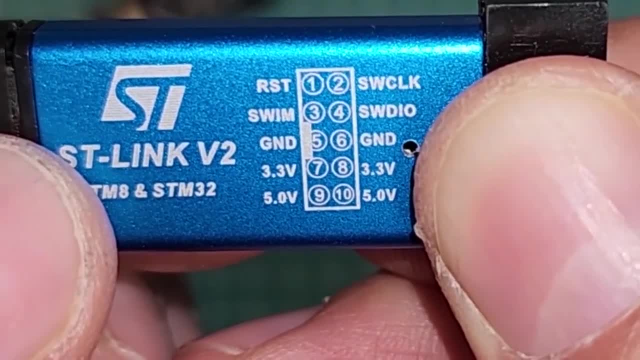 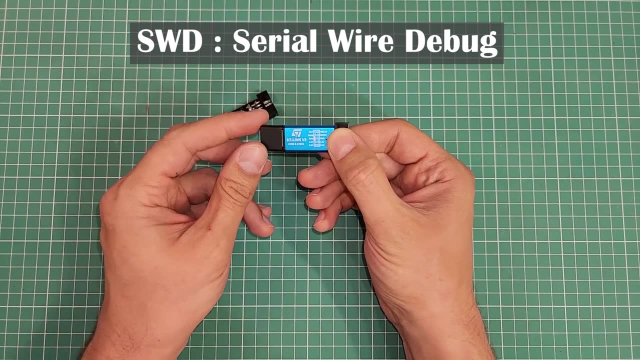 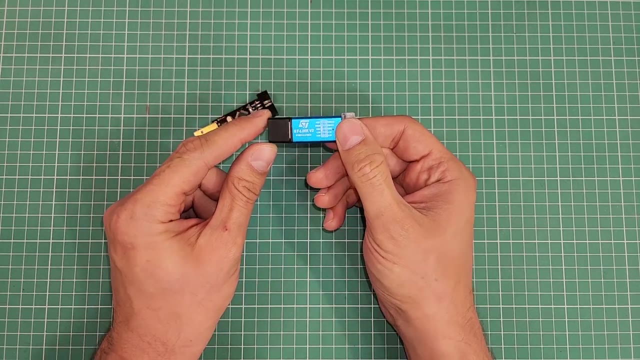 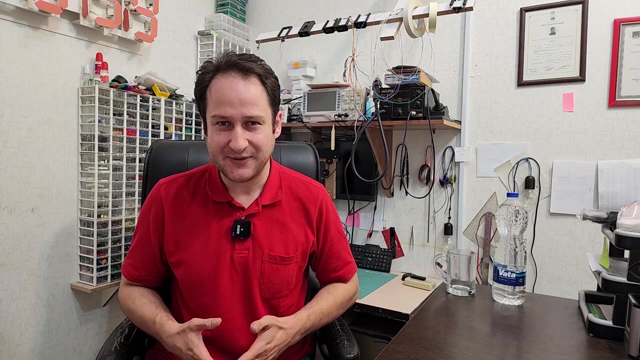 SWIM, SWCLK, SWDIO. These pins form the SWD protocol port. There are similar pins on STM32 microcontrollers. I will explain STM32 microcontrollers in detail in one of my next videos. Up until now, you have learned basic and general information about MCUs- Each MCU family. 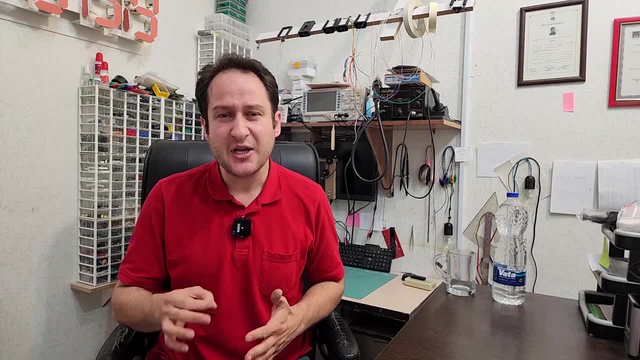 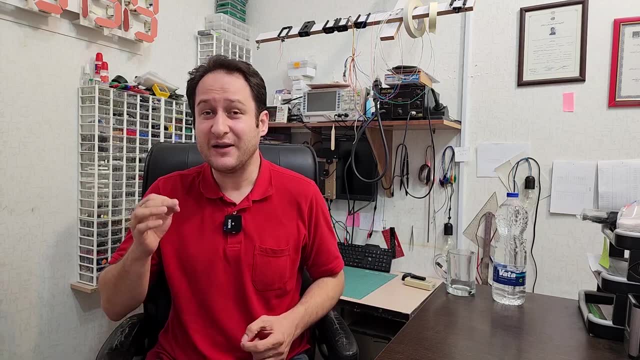 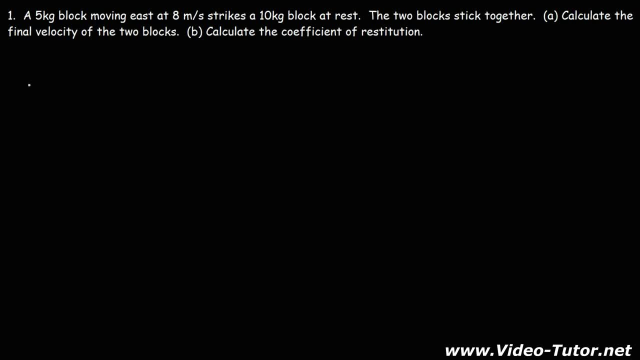 Let's talk about the coefficient of restitution. The coefficient of restitution is represented by the symbol e and it's equal to the ratio of the difference of the final velocities after the collision to the initial velocities before the collision. So it's equal to v1 prime minus v2. 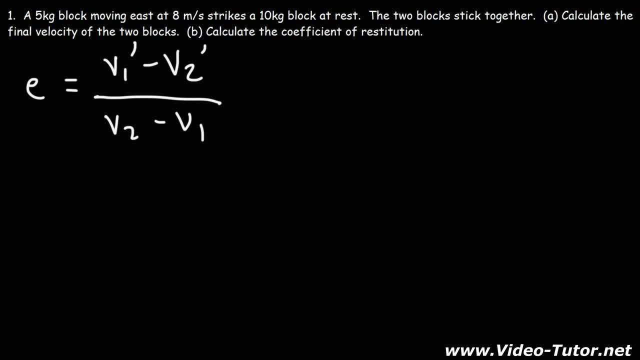 prime divided by v2 minus v1.. Now the coefficient of restitution. it's a number between 0 and 1.. When the coefficient of restitution equals 1, you're dealing with a perfectly elastic collision. Now, for all collisions, momentum is conserved.